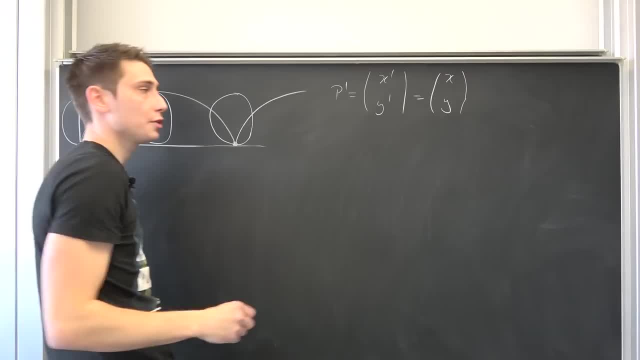 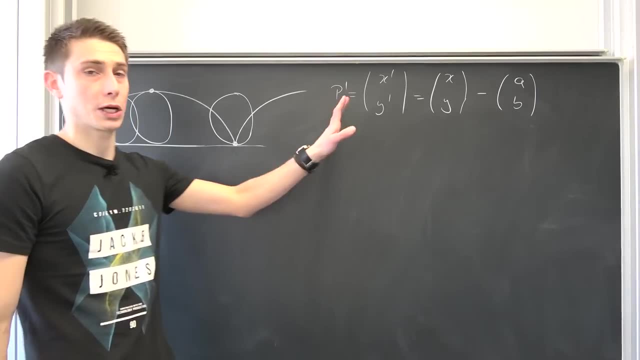 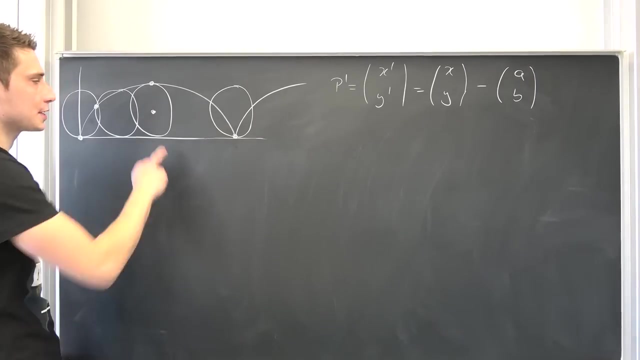 The coordinate of P in the original coordinate system, Minus a, B. if you don't know what I'm talking about, take a look at my cardioid video. I've explained it quite well there. Okay, at first I would like to find out where our Center is going to be all the time of the circle. 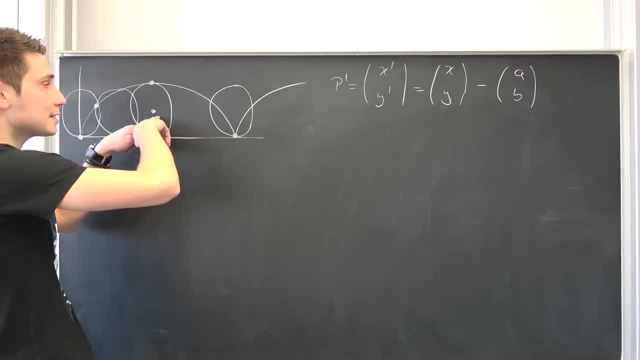 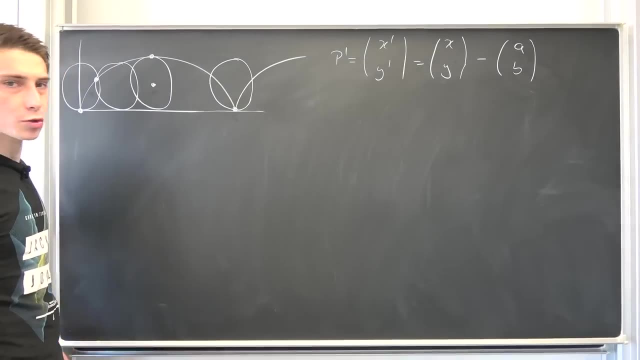 Because after that we can just place our new coordinate system in this very center and find out where our Point P P Prime is going to be in this new coordinate system all the time. So that's quite a powerful strategy. So we have to circle rolling. Here's our Center at the beginning then. 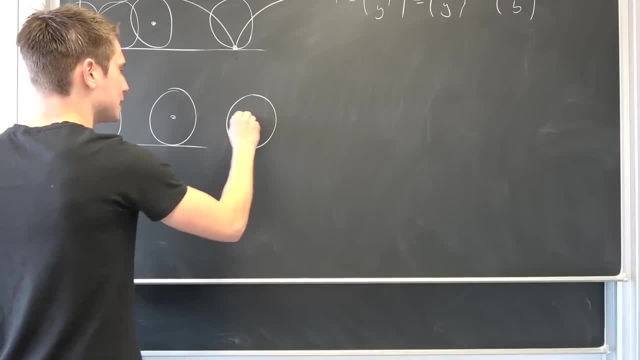 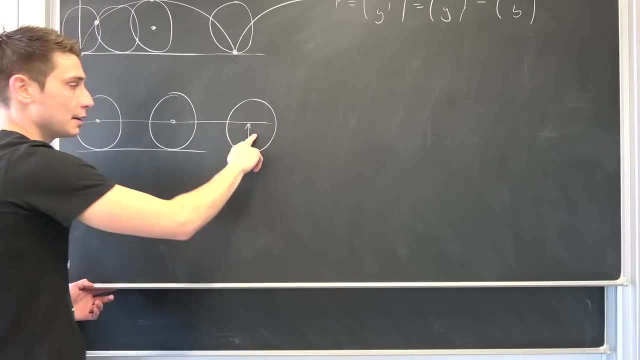 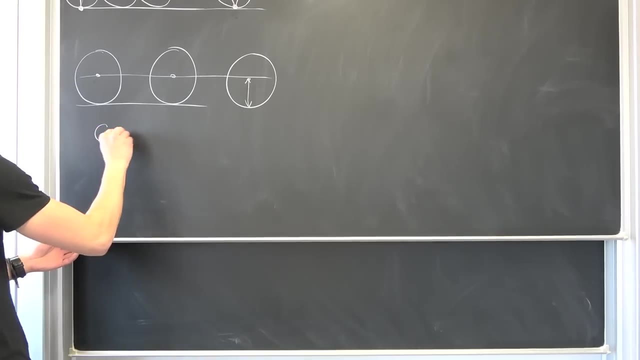 But further, here's our center, that then a bit further our centers here. meaning this really doesn't change: our Radius is going to stay the same all the time. meaning our is going to stay right on one new axis, you could say. Meaning our center is going to consist of some a and b coordinates, where our b coordinate. 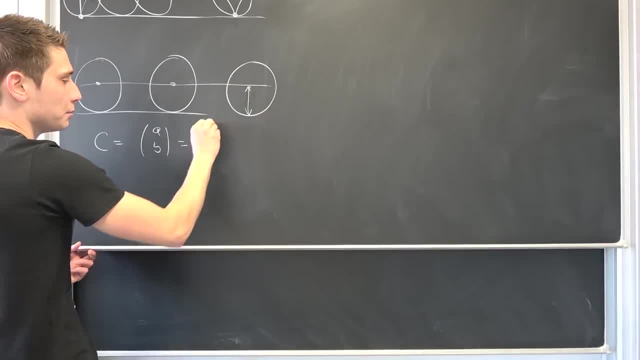 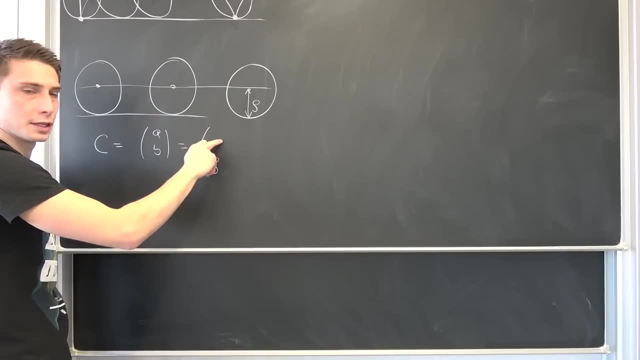 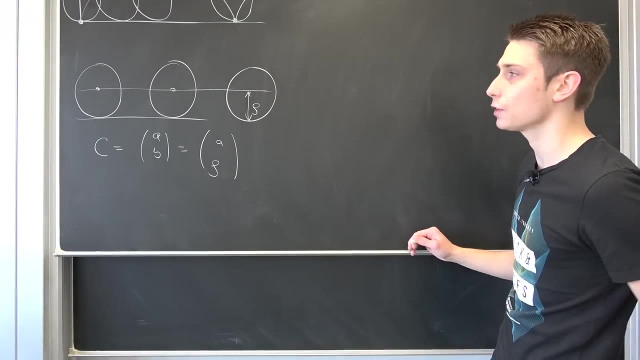 corresponds to the height where our center is, Meaning this is nothing but our radius, rho, r, whatsoever. Let's call it rho. But what about this up here, our x coordinate, What about that? Well, we can talk about this kind of intuitively actually, because, you see, at first our circle is somewhere here, then it's going. 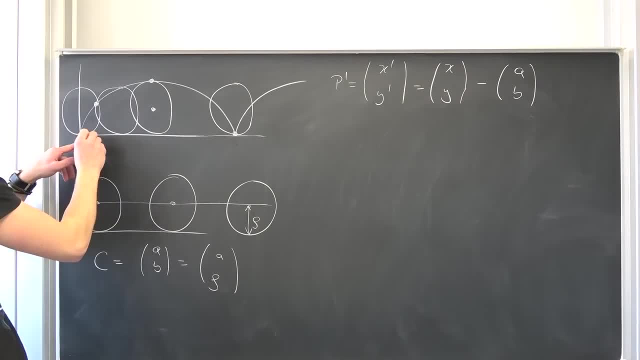 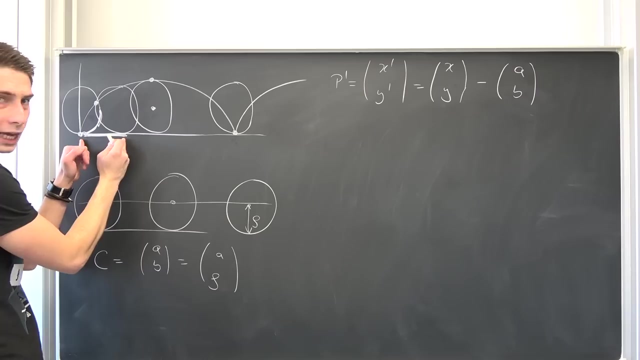 to roll a little bit Meaning. for example, if it rolls this distance right here, it corresponds to this part, for example, of our arc around the circle of our circumference Meaning. the length we have rolled is actually just a fraction of our circumference Meaning if our circle rolled. 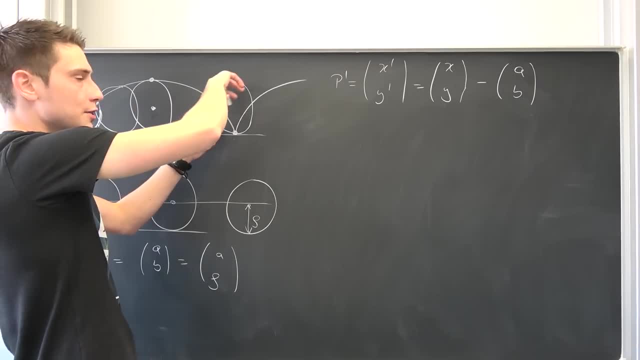 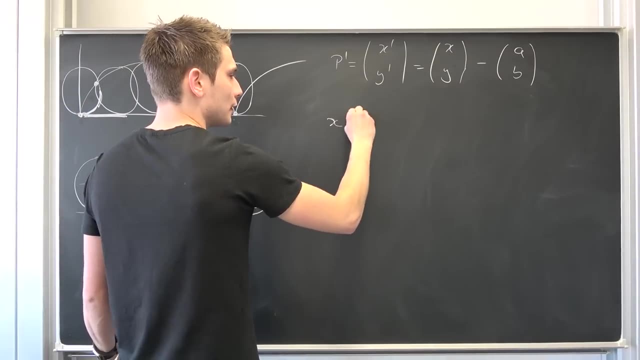 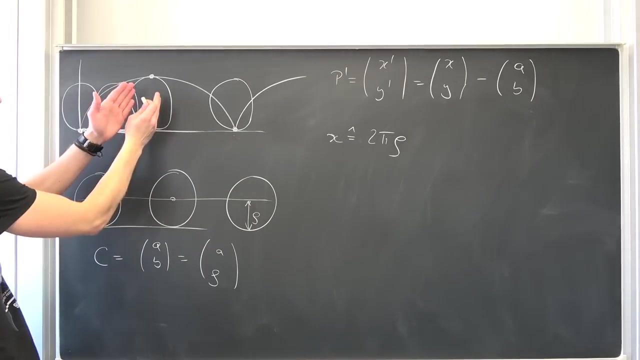 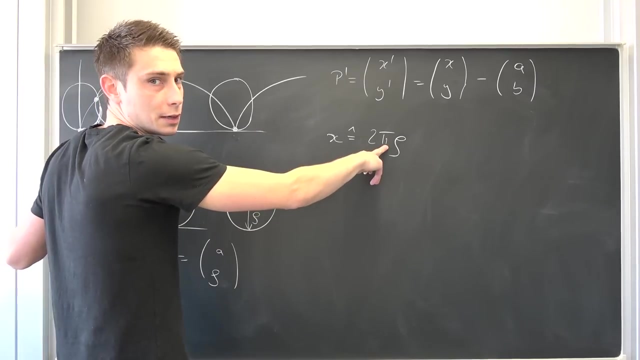 this completely. it has turned 360 degrees. 2 pi, meaning our x distance traveled, is going to correspond to, well, 2 pi times rho the whole circumference. if we just have half the distance traveled, well, then it corresponds to pi over 2. um, no, just pi times rho. 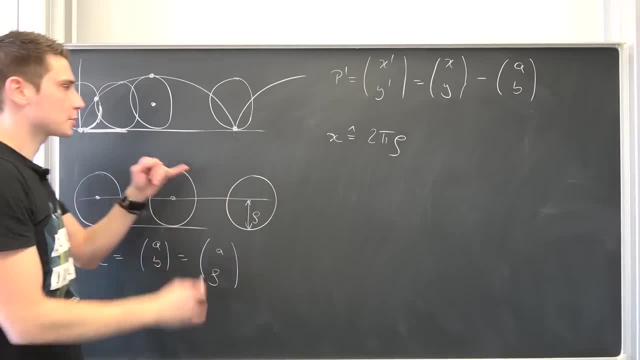 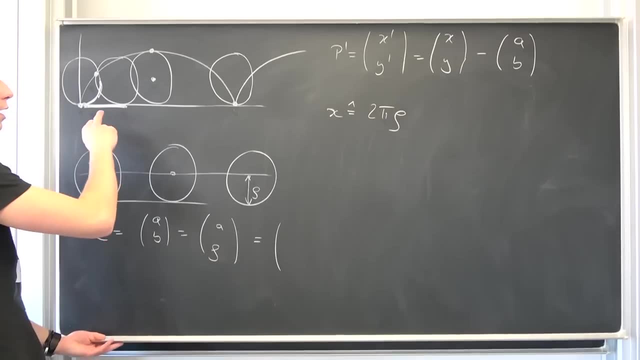 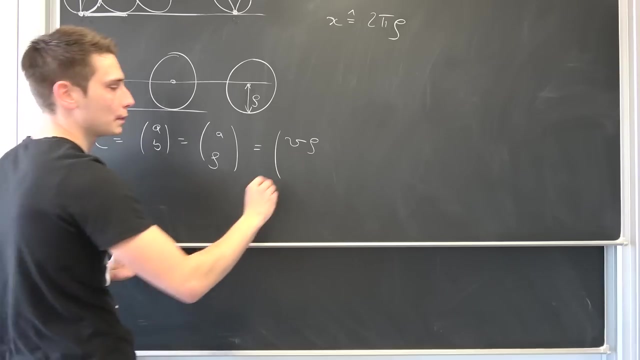 and so on and so forth. meaning this is just a formula for the arc length that you probably already know. our x coordinate is going to correspond to, well, our angle rolled. we are going to call it theta times our radius, rho, okay, and down here we have just our rho. i hope this. 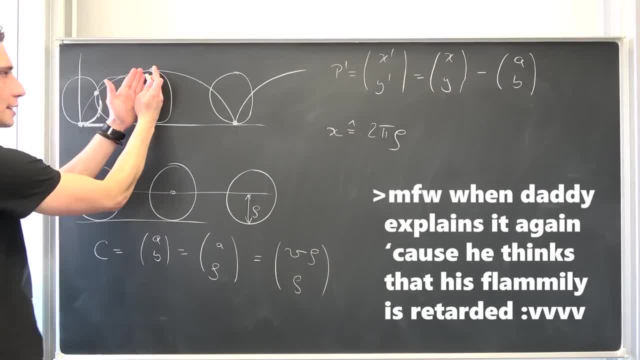 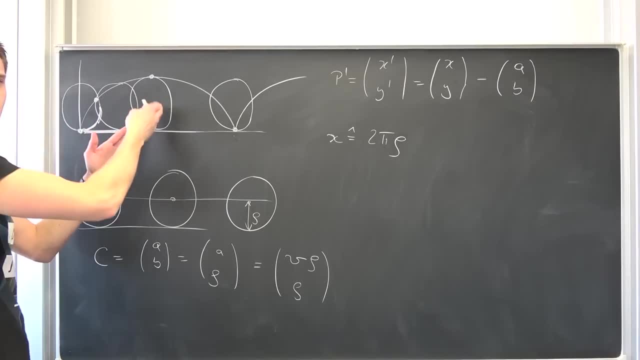 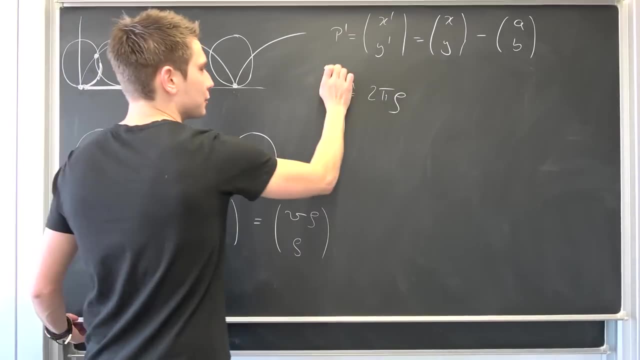 makes sense to you guys. so if our circle is in this position where our point is faced up right here, our point p, it has rolled 180 degrees, meaning our distance traveled is just going to correspond um. if this right here was our angle theta, okay, our rolled angle theta, and at this point it was 2 pi then. 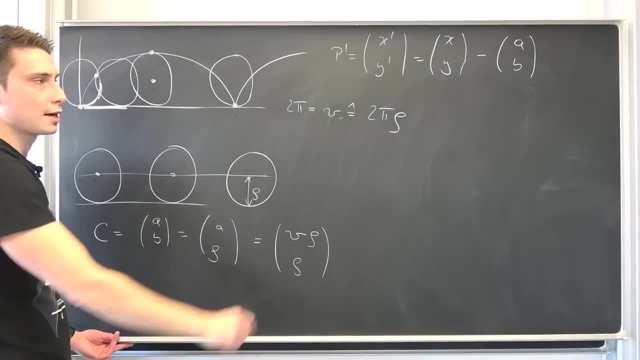 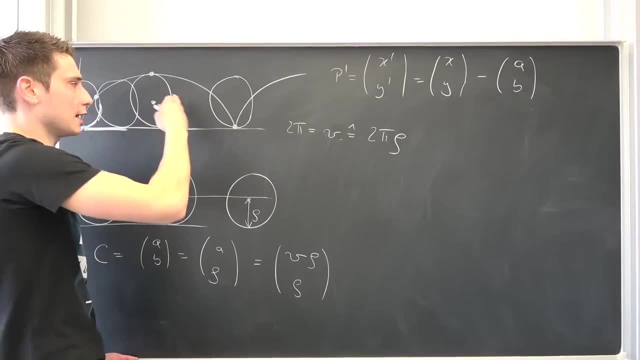 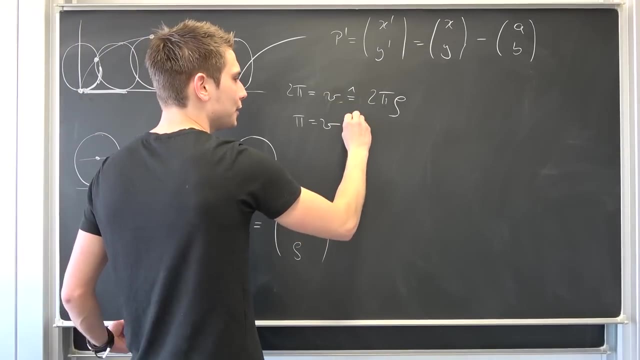 this corresponds to 2 pi times our radius rho. okay, i just want to explain it a bit further. but here, for example, if we just traveled half the distance of this cycloid structure, then our angle theta is nothing but pi, and it has rolled half the circumference, so meaning this is just pi. 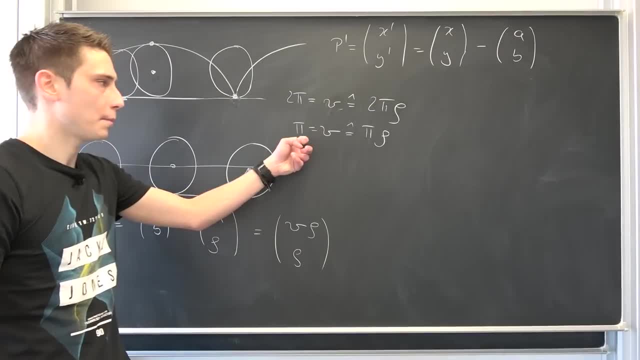 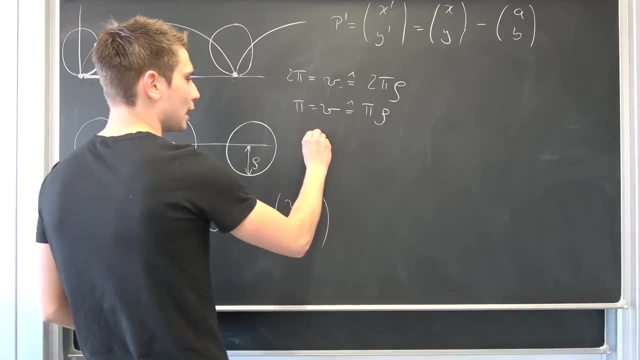 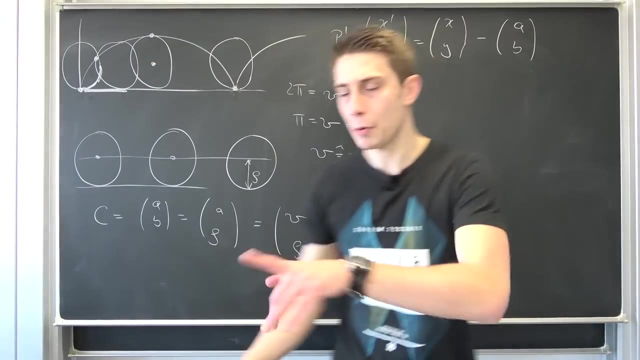 times rho. so you see, our angle theta pi corresponds to pi times rho. our angle theta 2 pi corresponds to 2 pi times rho, and so on. meaning our angle road corresponds to theta times rho. what do we have down here now? we have fun, found out where our center is actually all the time, meaning we can. 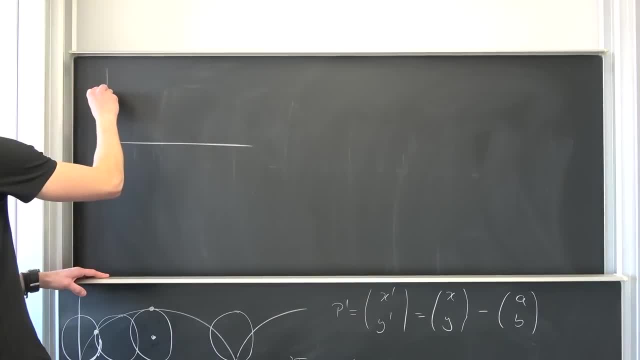 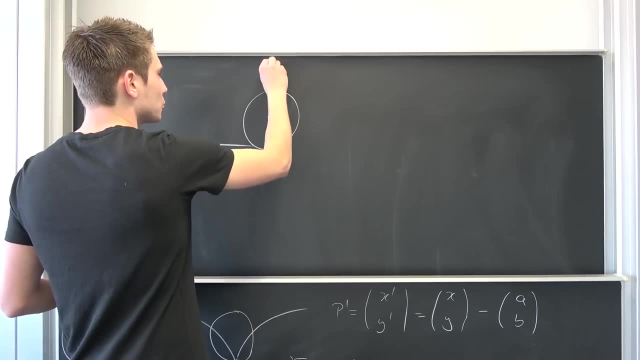 go from here to this point, and then we have to find out where our center is actually all the time, meaning we can place our new coordinate system somewhere. so this was our initial position. okay, that's fine, then. it has rolled quite a lot. now it's here, our circle, and now we are going to place a new coordinate. 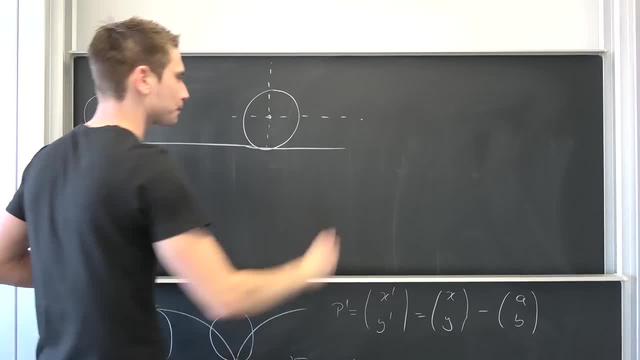 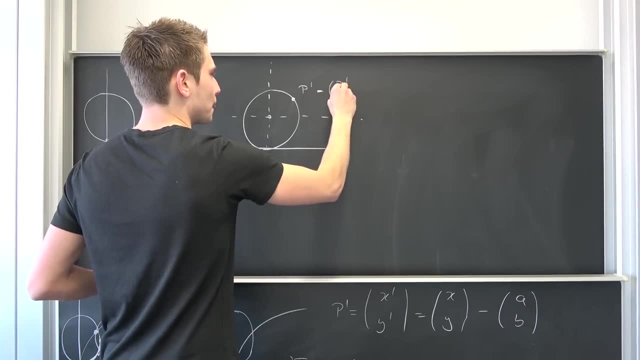 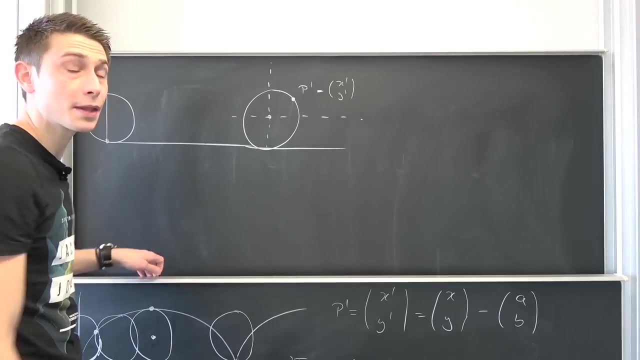 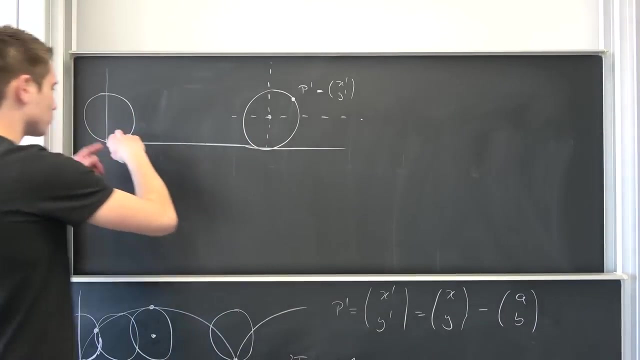 system in here. okay, this is our new point: p prime with an x prime and y prime coordinate. okay, it has rolled pretty far. you can take a look at many different situations right here. what is our rolled angle that we actually have? well, our angle that we have rolled up until now is, from start, meaning. 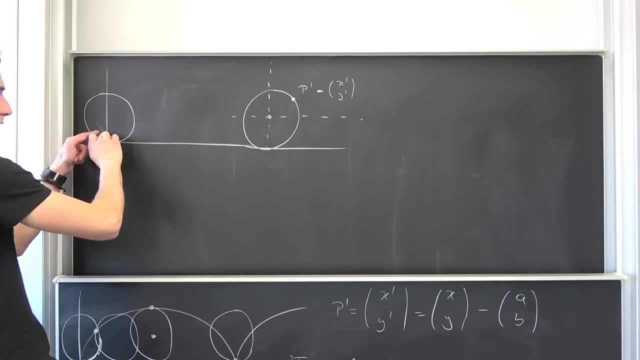 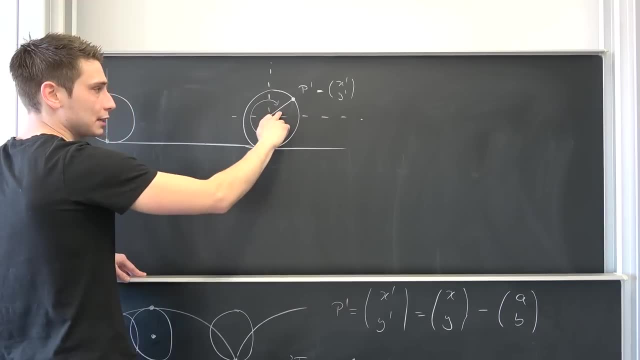 it lies here somewhere. so here it has rolled zero degrees, but right here it has rolled this distance, right here where we can just connect this as being a vector, our p prime vector in this new coordinate system. so it has rolled up until here. this is our robot angle fader. 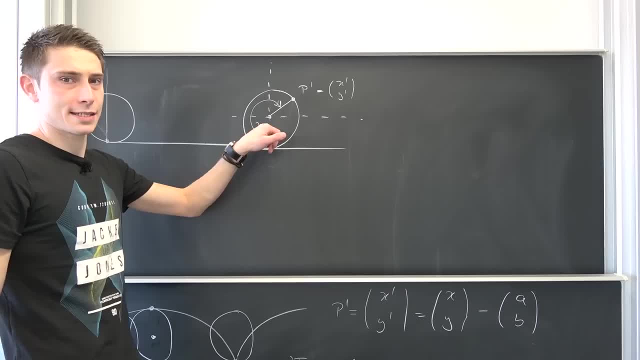 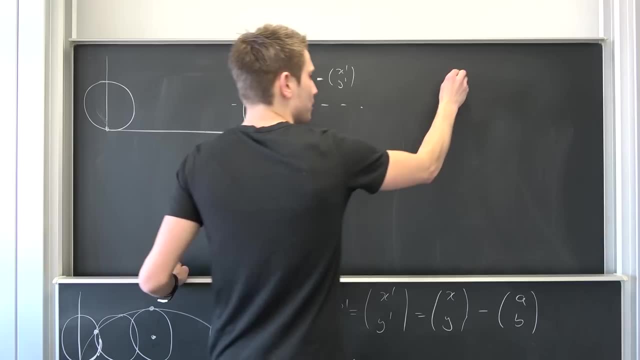 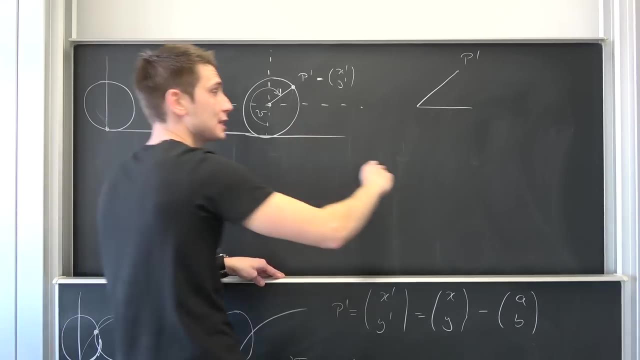 and I can. then we curry going to this new coordinate system. so I could say this vector p is value of125 and then let's say my Theresa is value is being vaulted into that, my BTS signal. so I can add a line up there. I'm going to rank this and then move the value up to 25. 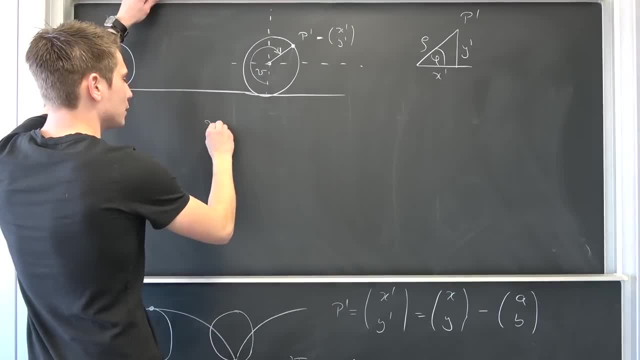 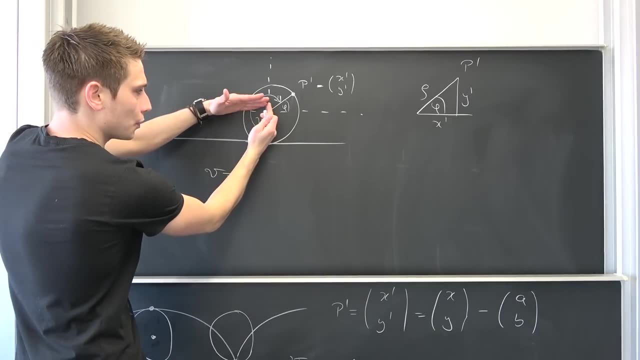 how can we make sense of this fader? what is this fader all the time in this new coordinate system? Then our angle theta that we have is nothing but okay. if this right here is our phi, then this quarter right here is just pi over 2, 2, pi over 2, 3, pi over 2.. 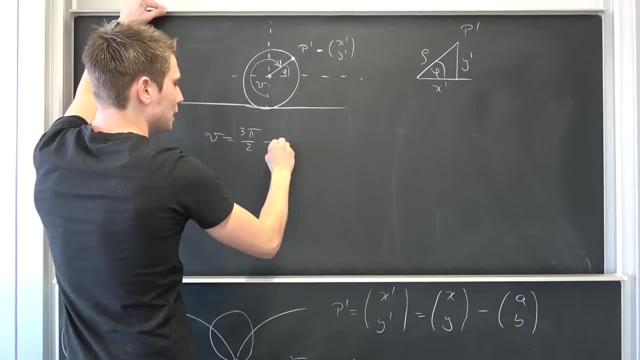 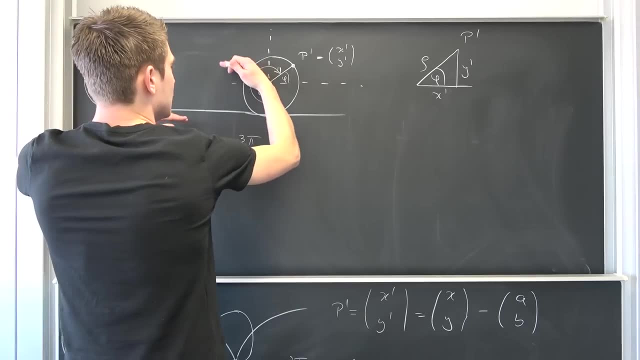 So this is nothing but 3 pi over 2 minus phi. This is going to be our angle, rho, that we have right here in this situation, And you can do it differently. You can work with this quadrant right here or this quadrant right here. 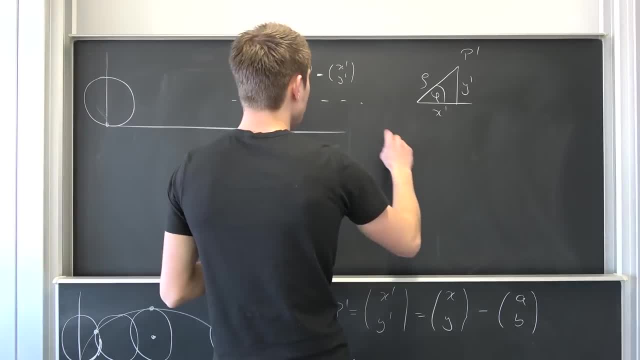 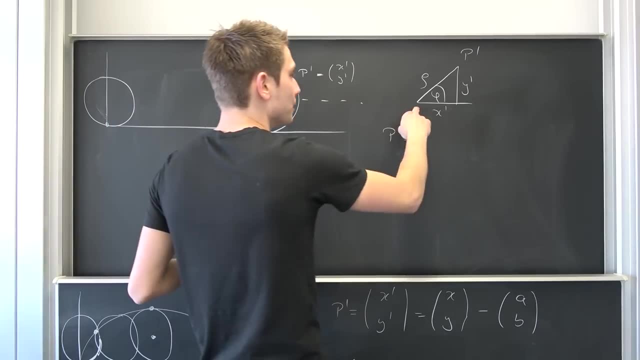 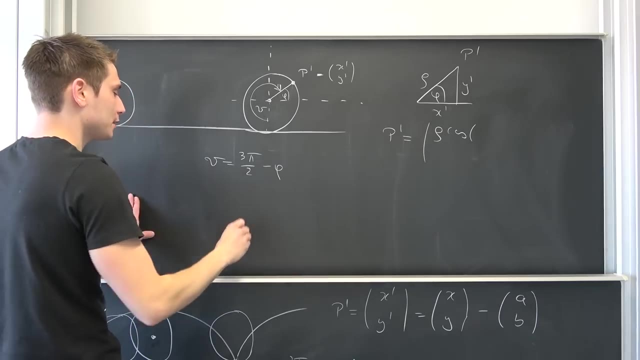 Okay, our p prime is going to be, if we use Papa-Pi-Fagoras, nothing but okay. x prime, y prime, coordinate, meaning it's nothing but rho times the cosine of phi. but phi is nothing but 3 pi over 2 minus theta. 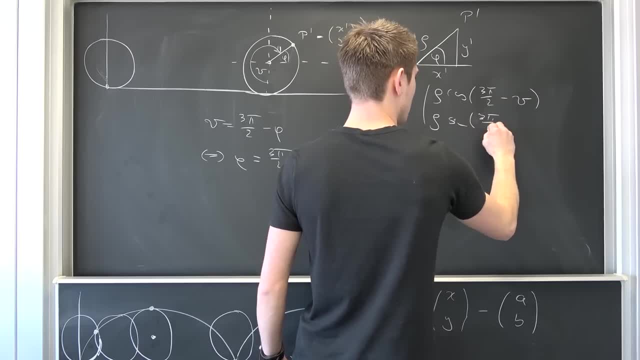 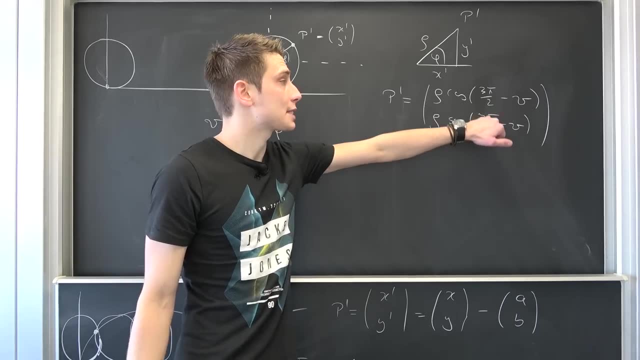 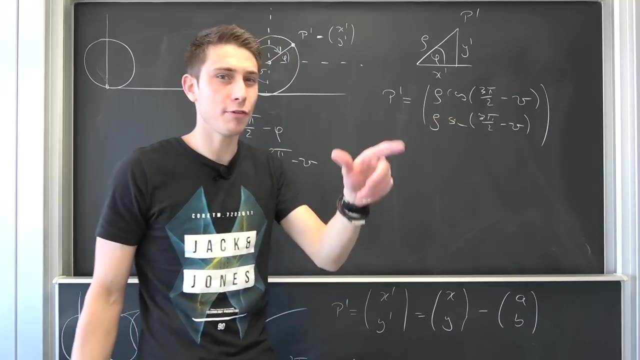 Same spiel, Same spiel, Same one here, Just with the sine this time. Okay, coolio, You can break this up into the real and imaginary part of the complex exponential function. Overall, you can factor out this e to the i: 3 pi over 2.. 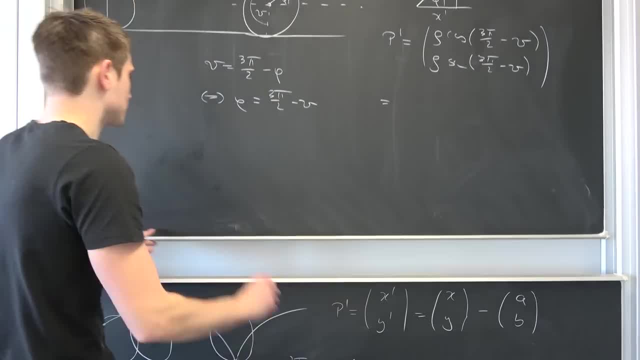 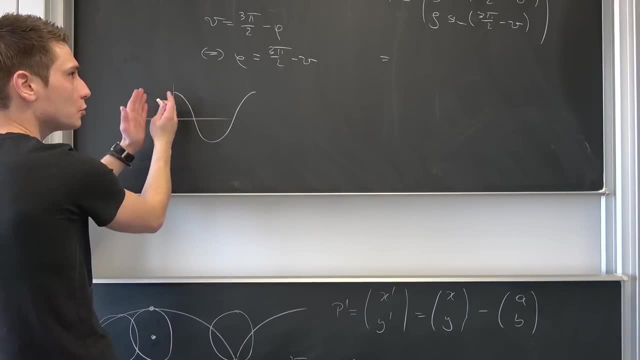 And you are going to notice this is just a shifted sine wave. So you can also take a look at this graph right here for the cosine. This is it in the normal case. If we shifted pi over 2 to the left, it's going to be this thing right here. 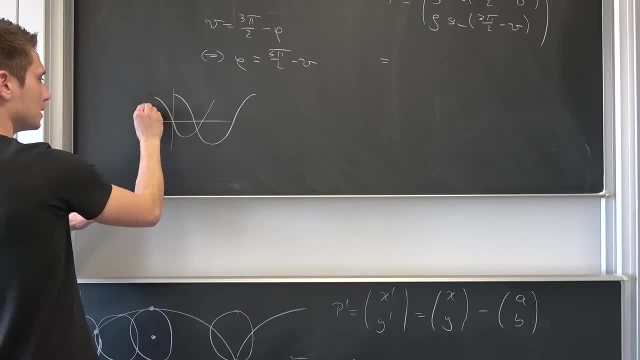 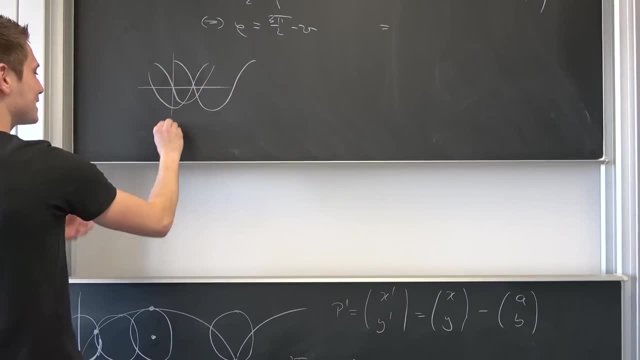 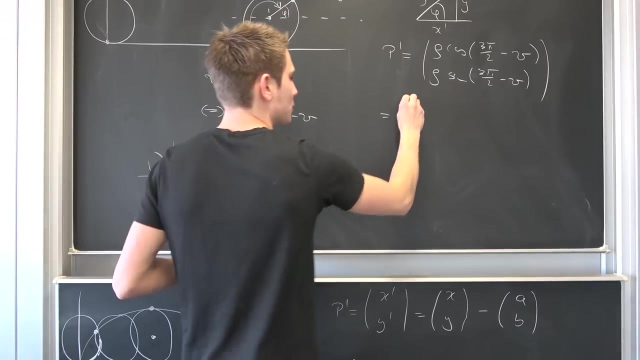 If we shifted pi to the left, it's going to be negative cosine, And if we shifted more pi over 2 to the left, it's going to be nothing but this right here, the sine in this case, So it's going to be rho times the sine of negative theta. 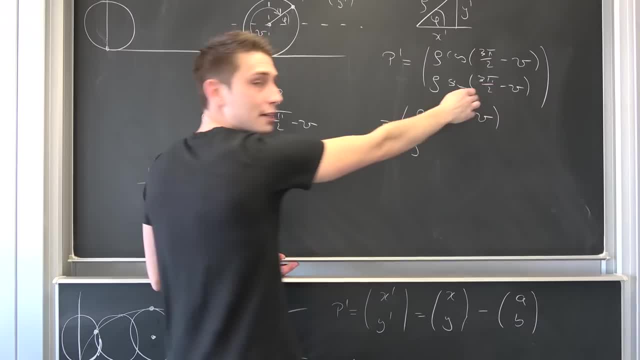 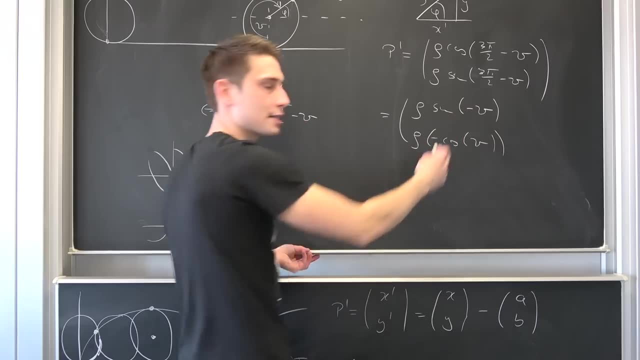 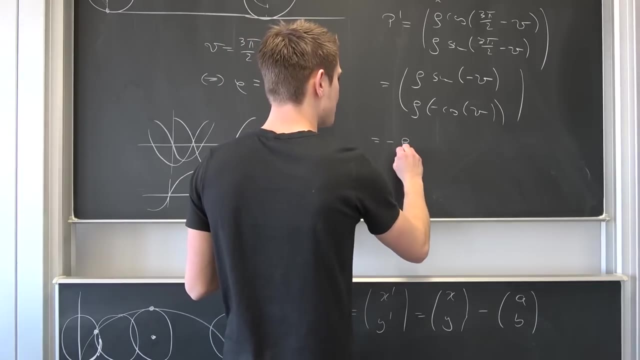 And down here it's going to be rho times here. in this case it's the negative Cosine of theta. Sine of negative theta is nothing but negative sine of theta. So we are going to get common factor of negative rho that we can bring to the outside. 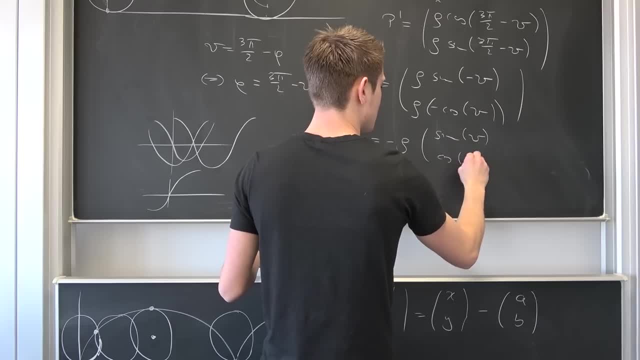 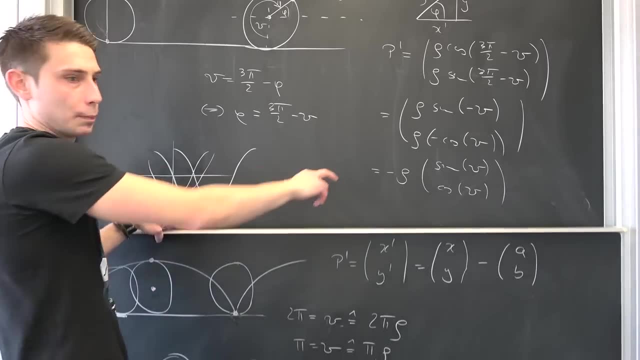 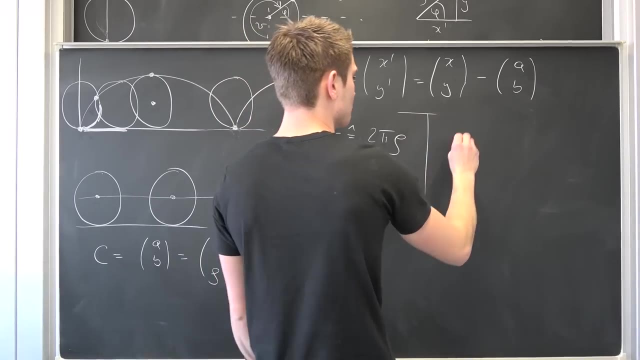 And then we have the sine of theta and this cosine of theta vector, And then we are already done because we have found out where our p prime is, all the time Meaning we can just solve for our point p initially right here In this initial coordinate system, meaning our point p consisting of an x and y coordinate. 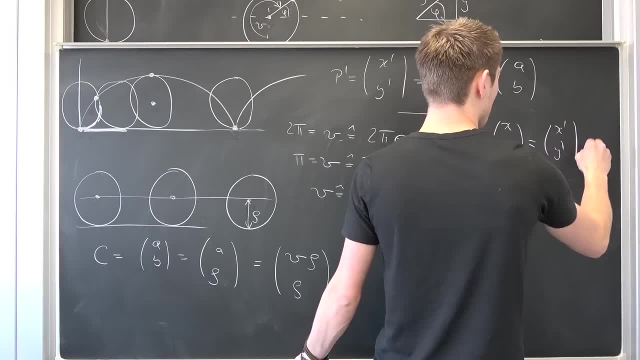 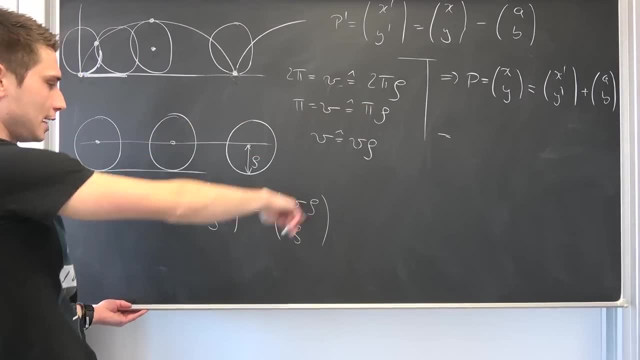 is nothing but well, x, prime, y prime plus a, b, And we can just plug this chunk into here that we have gathered. So a and b is nothing but okay. we have a common factor of a common scalar of rho, rho. 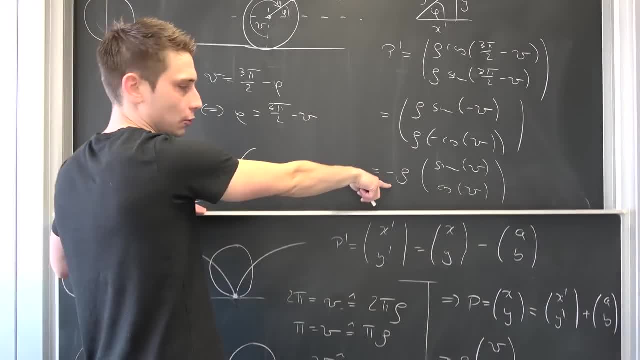 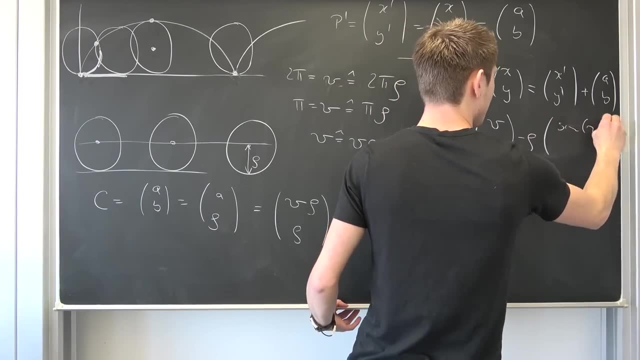 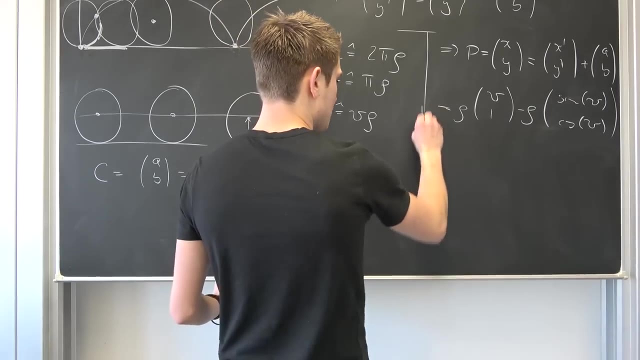 theta 1, and then positive. okay, it's going to be negative right here. Negative rho, Sine of theta, cosine of theta. If you want, you can factor out some more stuff. So for example, this rho, right here. 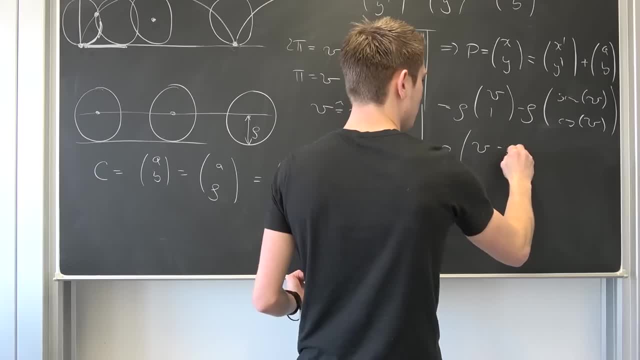 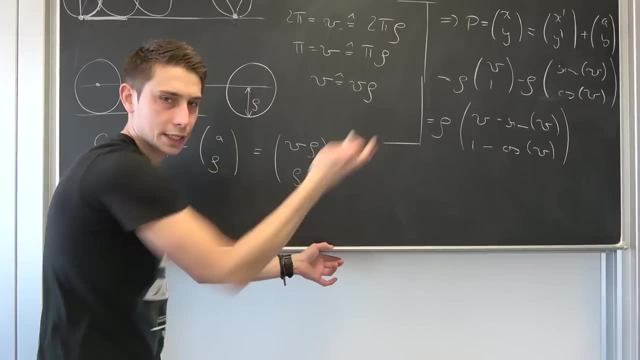 So this is nothing but rho, And then we are going to get theta minus sine of theta, And then we have 1 minus the cosine of theta. Whatever you do, this right here is our answer, And I thank you guys for watching. 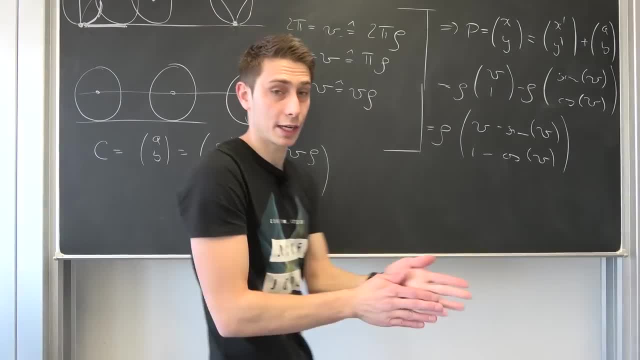 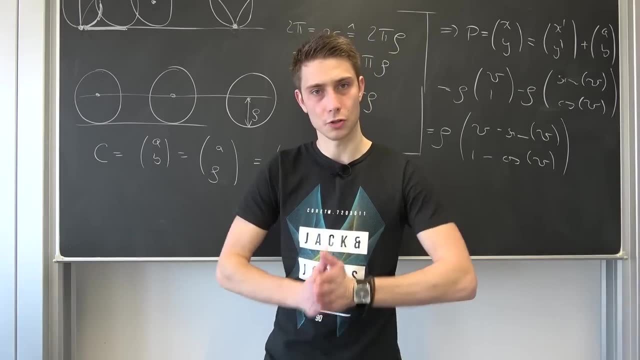 If you did enjoy this video, please like and subscribe and recommend the channel, if you like. If you want to support the channel a bit more, you know how you can do it: Just buy those t-shirts I created. This is not one of them, but I think it looks quite good on me. 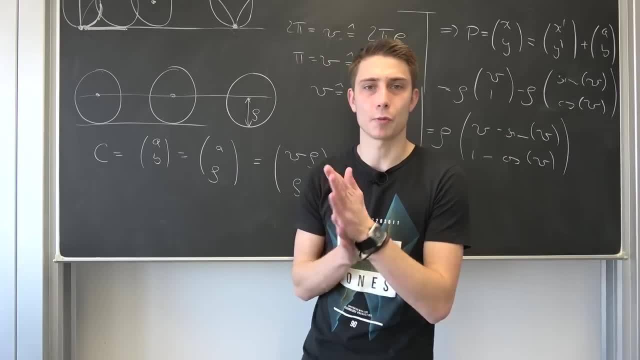 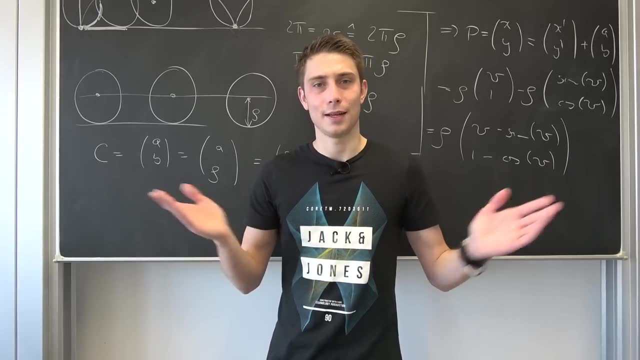 It fits me so well. just like with most of the stuff that I'm wearing, I'm only wearing the stuff that I'm feeling comfortable in. Anyways, what else can I say? Thank you guys for watching and I love you guys.